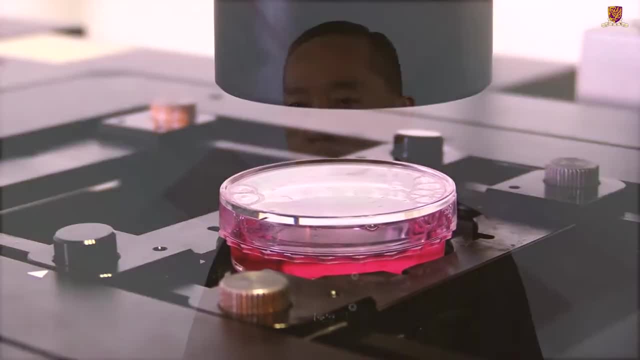 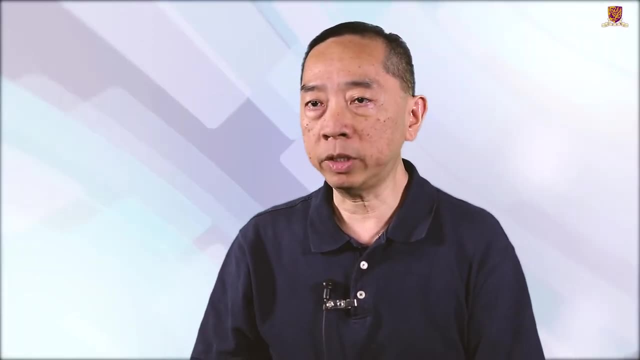 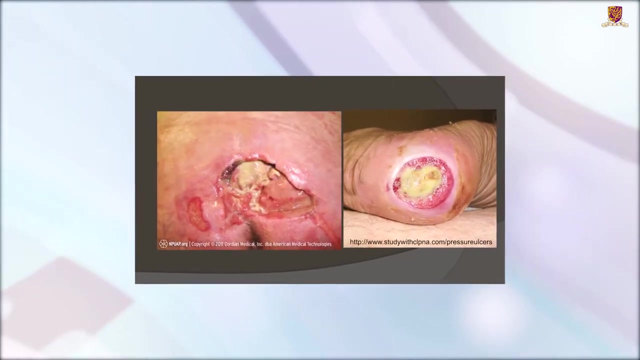 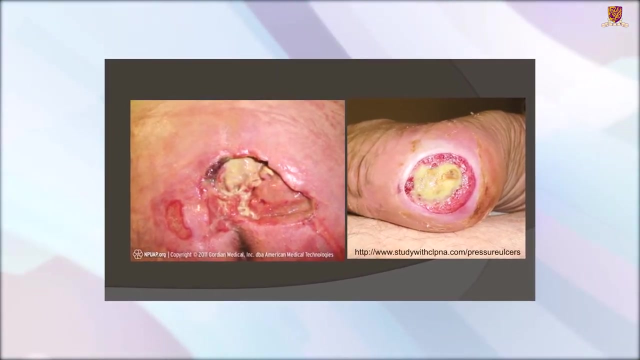 houses when body tissues are subjected to moderate but prolonged mechanical stresses, and how to design body support interfaces To reduce the risk of such houses. Such houses arise from localized injury to the skin and all the underlying tissues, usually over a bony prominence, as a result of pressure. 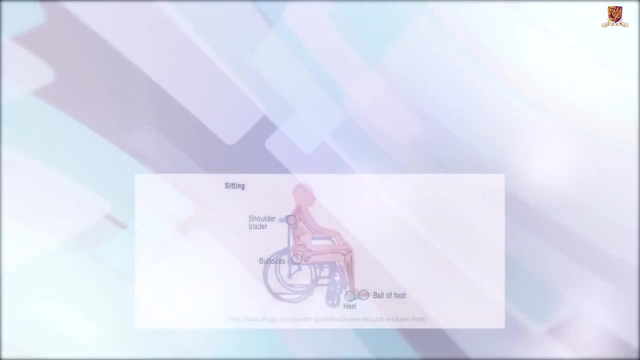 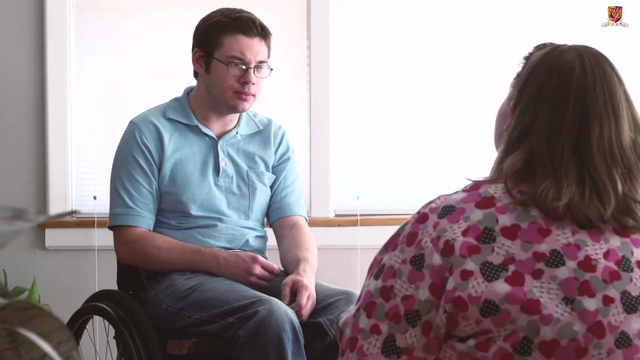 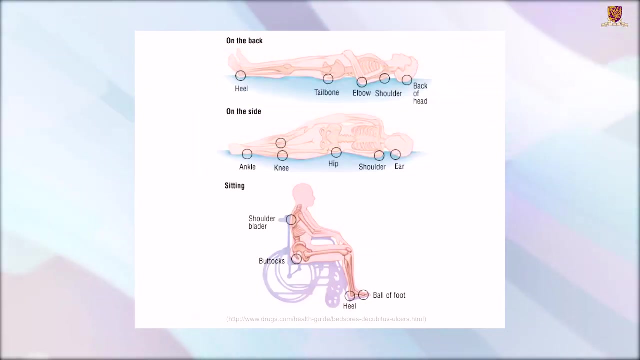 or pressure in combination with shear. My research interest is motivated by the clinical challenge faced by many people with disabilities, like a person with spinal cord injury who needs to sit on wheelchair for a long time. like a frail elderly person who needs to rest on. 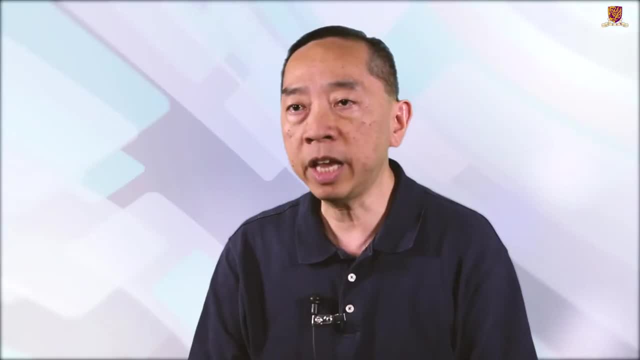 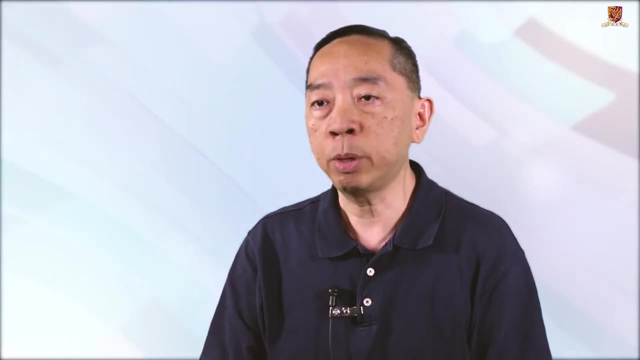 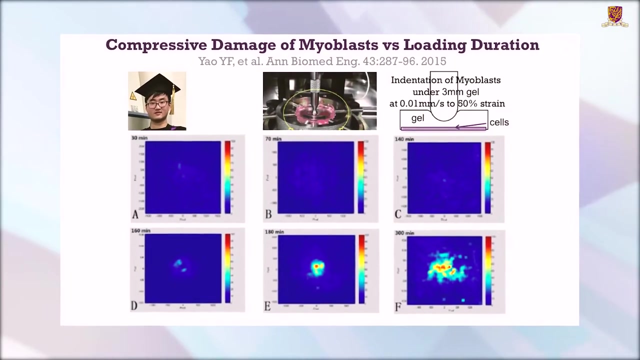 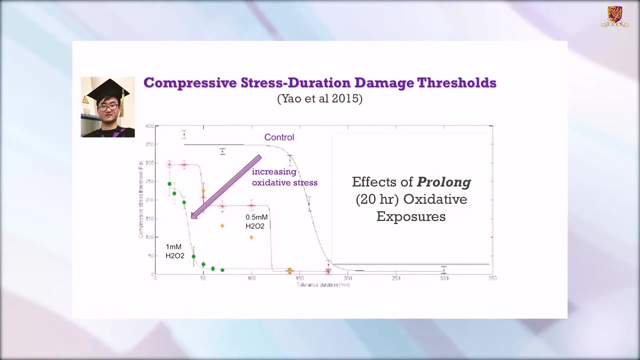 bed most of the time. In recent years, my students and I have launched a series of multi-scale studies on deep tissue injury under prolonged biomechanical and biochemical stresses. We assessed the duration-dependent damage thresholds of muscle cells under mechanical stresses. Both support the hypothesis that chronic exposure to high-dosage oxidative stress could compromise. 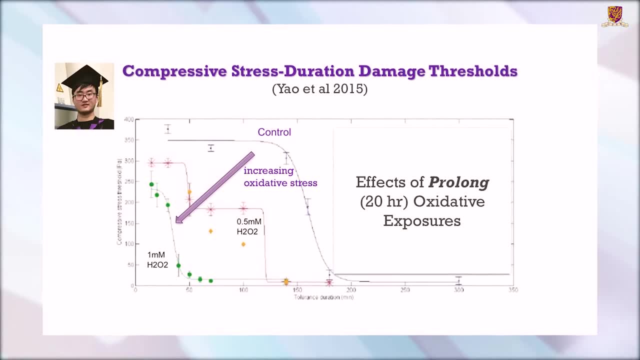 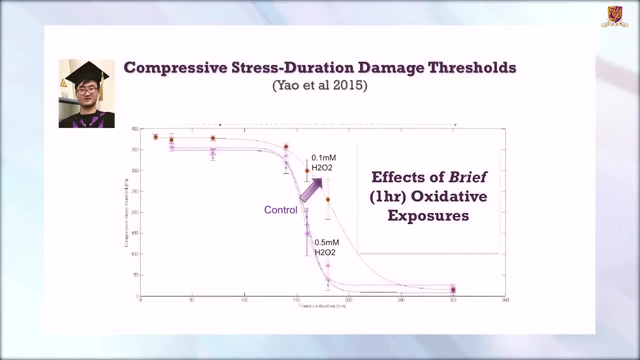 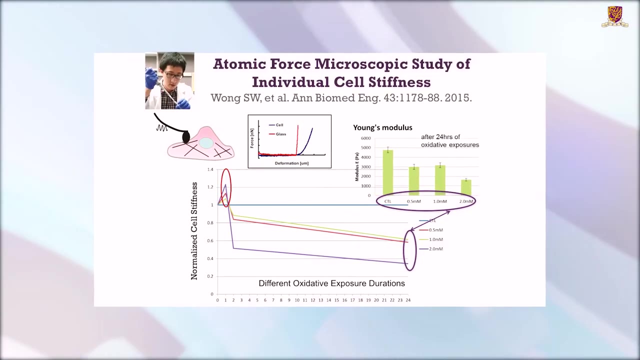 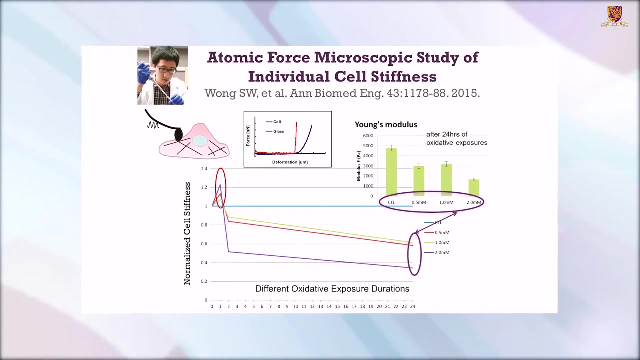 the capability of muscle cells to withstand mechanical damages, while short exposure to low-dosage oxidative stress could enhance such capability. We examined the effects of oxidative stress on cytoskeletal actin polymerization and used an atomic force microscope to monitor the corresponding temporal changes in cell stiffness. 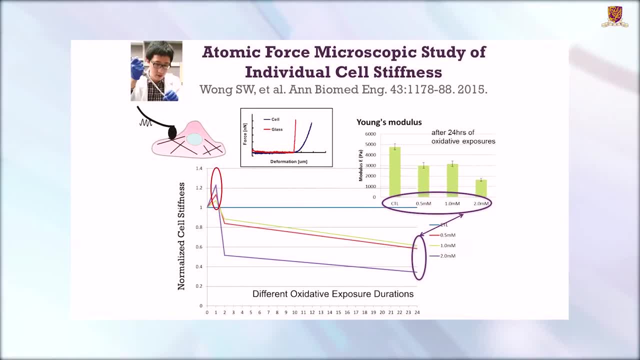 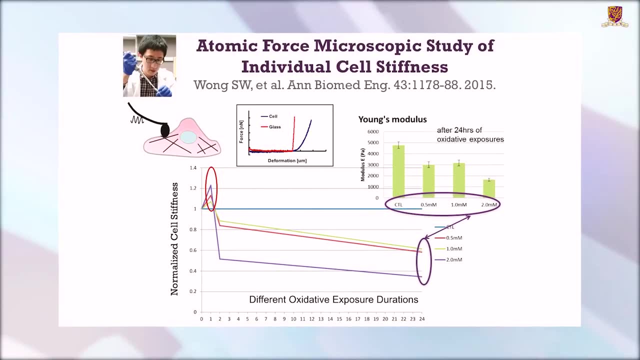 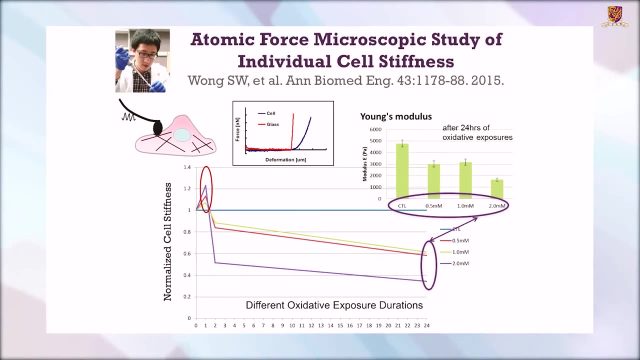 Atomic force microscopy results show that short exposures to oxidative stress apparently increase the stiffness of microtubes, but that long exposures make the cells softer. The turning point seemed to take place somewhere between one hour and two hours of oxidative exposure. Thank you for watching. 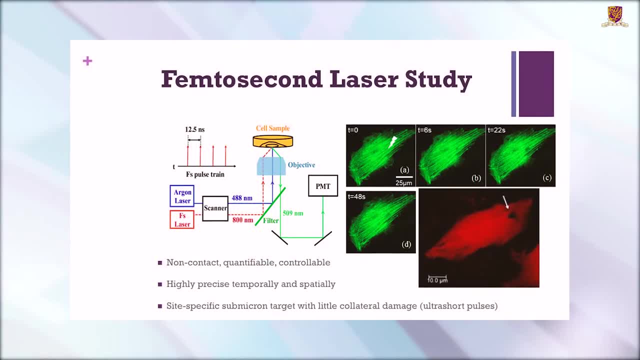 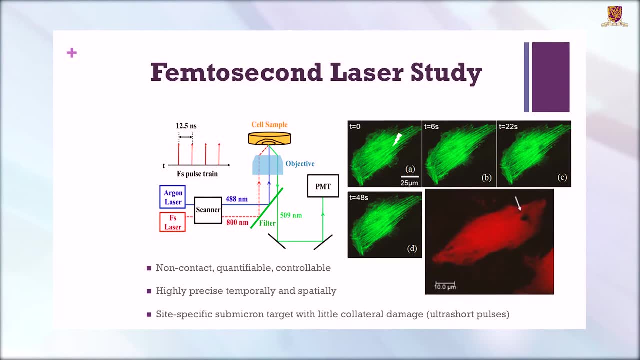 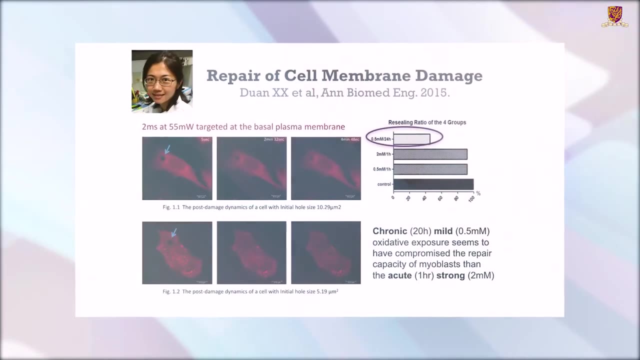 See you next time. We used femtosecond laser to evaluate how oxidative stress affected the pre-tension in the cytoskeletal fibers and the ability for cells to repair a micron-sized pore on the plasma membrane. We also find that mild but chronic oxidative exposure seems to have compromised the repair.